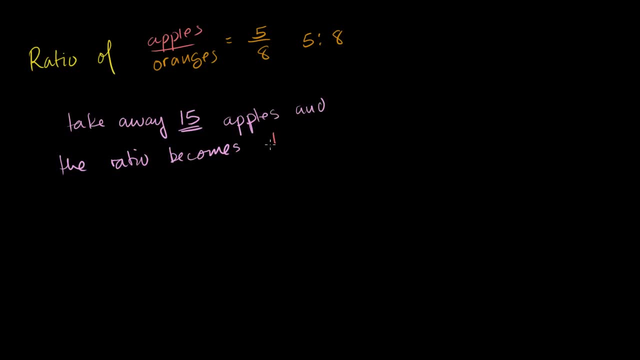 The ratio of apples to oranges becomes 1 to 4.. How many apples? How? Let me write it this way- How many total, not how many apples. let me say how much total fruit instead of how many fruit. How much total fruit do I have after taking away the 15? 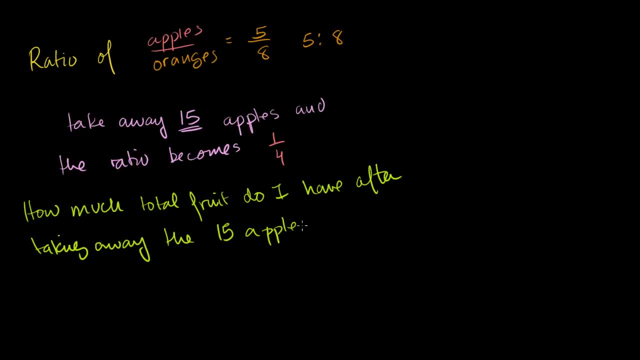 apples. How much total fruit do I have after taking away the 15 apples? How much total fruit do I have? So let's do a little bit of algebra. Let's say that x is the number. x is equal to the number of fruit that we start with. 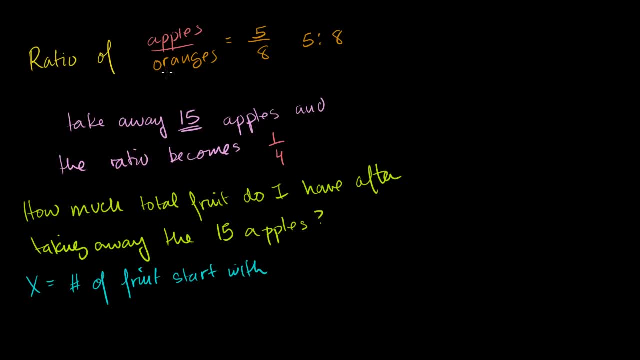 How much fruit are we going to end up with at the end? We're taking away 15 apples. We're not doing anything to the oranges, so we know that: x minus 30.. I'll do that in a second. I'll do it in a different color. 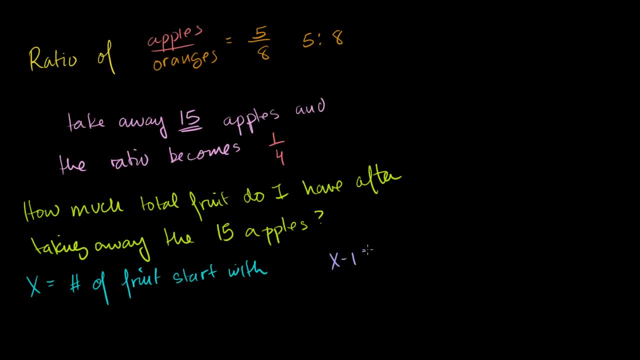 x minus 15.. We take away 15 apples. x minus 15 is equal to the number of fruit we end up with. We know these two things are true, And now we know that we start off with a ratio of 5 to 8.. 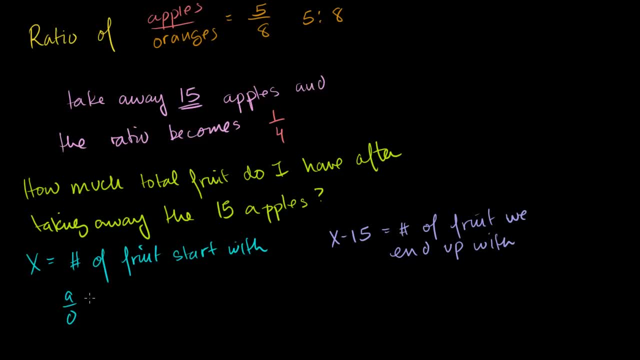 So we know that the ratio of apples to oranges is equal to 5 to 8. That we start off with- Or that's just another way of saying that- for every group, assuming that we can divide our group of fruit into a set of groups and every group has the same number of apples and 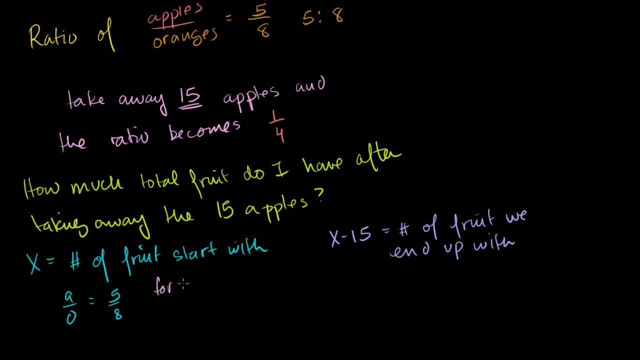 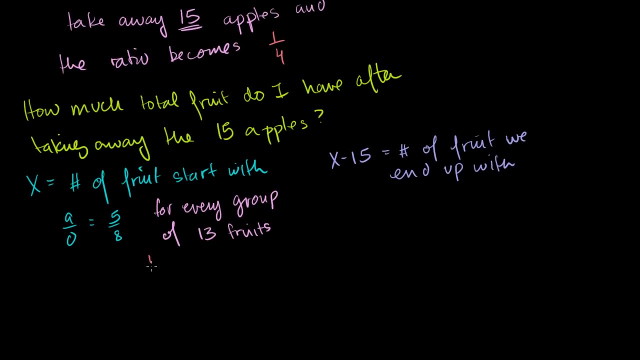 oranges. that means that for every group of what 13 fruits, there are 5 apples and 8 oranges. That's what this tells me. For every group of 13 fruits, there are 5 apples and 8 oranges. 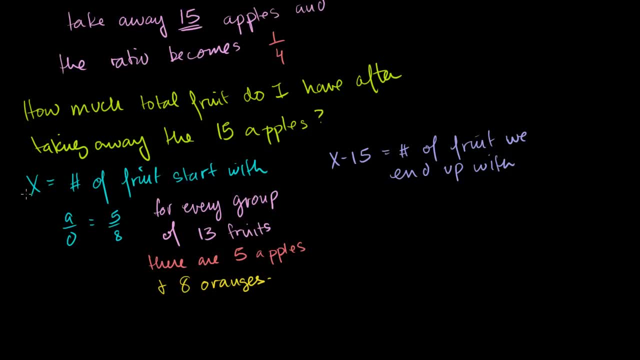 And how many groups of 13 fruit are there? Well, I have x total fruit. So if I divide x divided by 13. If I take x divided by 13. That is equal to this is the 13. right here I have 13 fruits. 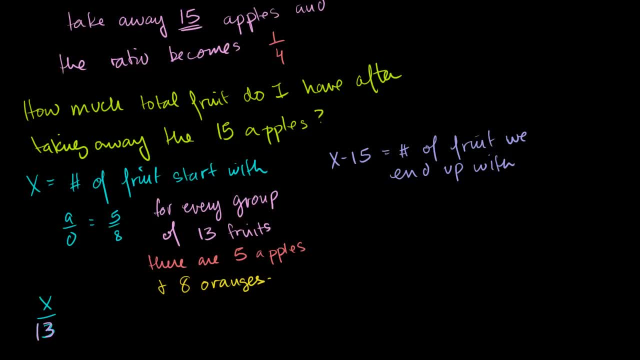 per group I have x total fruit. so this is the total number of groups. So this is equal to the number of groups. Now, for every group, I have 5 apples, So how many apples am I starting off with? This is the number of groups. 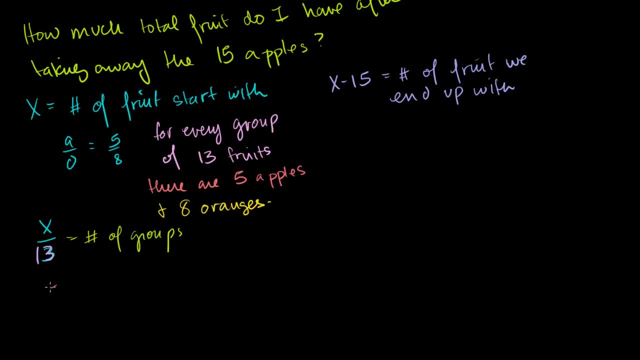 For every group I have 5 apples. so I'm starting off with 5 times that apples, 5x over 13 apples Now for every one of these groups I also have 8 oranges. So how many oranges do I have? 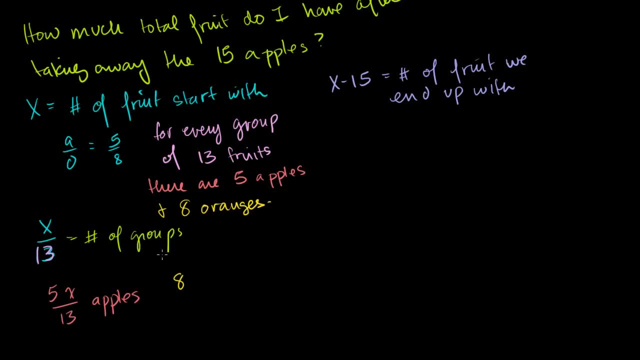 I have 8 times that, Because for every one of these I have 8 oranges. So 8 times that is 8x over 13 oranges. Fair enough, That's what I start off with Now when I'm done. we said that the ratio of apples to 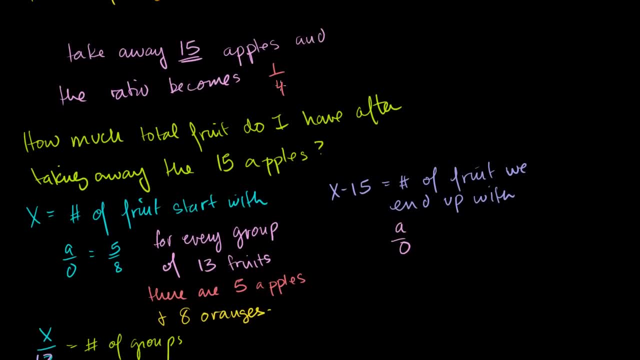 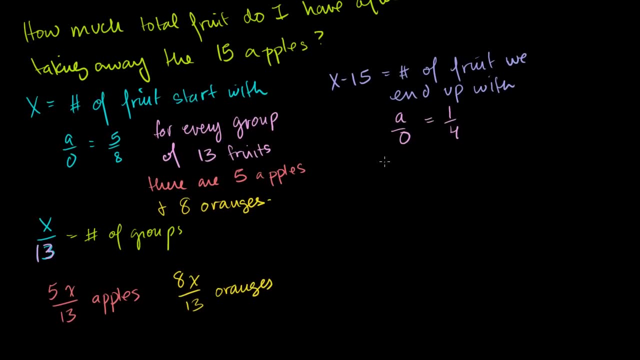 oranges, The ratio of apples to oranges becomes 1 to 4.. Becomes 1 to 4.. Or another way of saying that is that for every 5, if you add these two numbers together- for every 5 fruit there are 1 apple and 4 oranges. 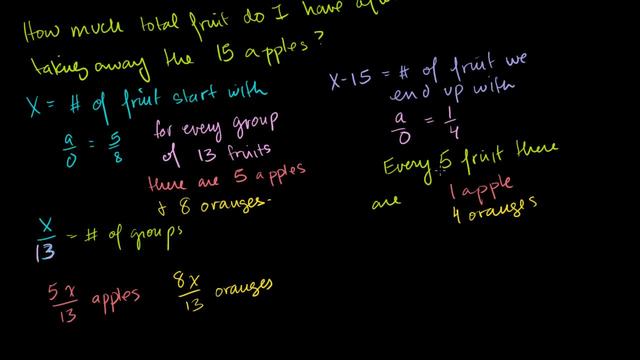 Fair enough. So how many groups of 5 fruit do we have? Well, this is the total number of fruit we're left with if we took 15 away. So how many groups of 5 do we have? We take the total number of fruit x minus 15, divided by: 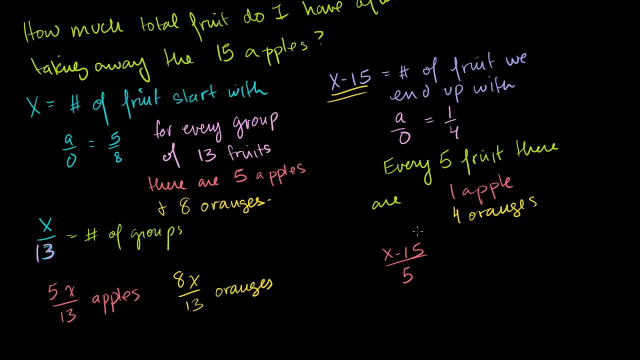 how many fruit we have per group, And this is how many groups of this is equal to the groups of 5 fruit, Of 5 fruit Now, For each of these groups, we have 15.. For each of these groups, I'm going to have 1 apple and 4. 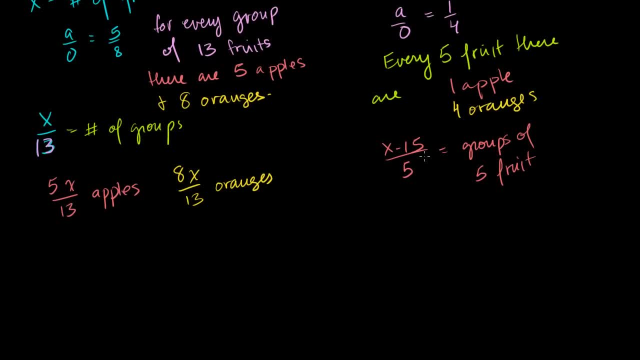 oranges. So how many apples and oranges do I now have? after I took away 15 of the apples, I took away 15 fruit. So let's think about this a little bit. How many apples am I going to have? I have 1 apple for every one of these groups. 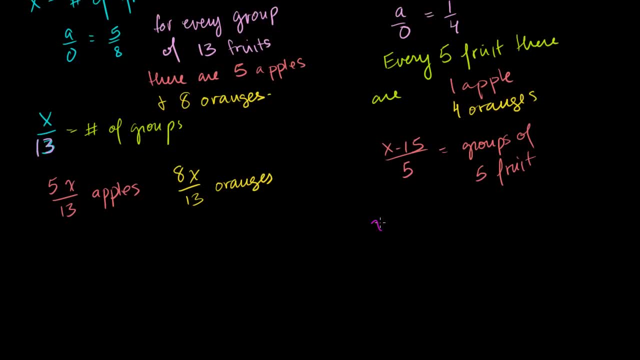 So that's how many. so the number of groups is the number of apples I have. So I'm going to have x minus 15 over 5 apples. And then how many oranges am I going to have For every one of these groups? 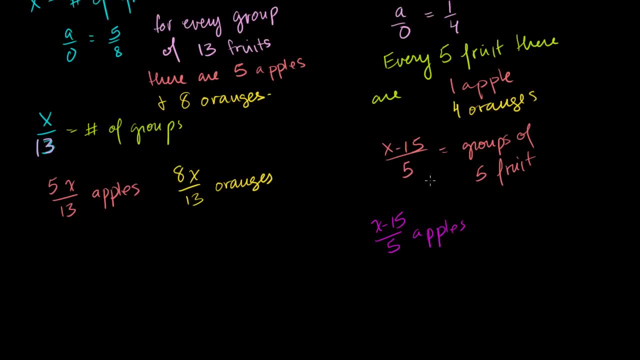 I'm going to have 4 oranges. So I'm going to have 4 times this many oranges. So we could write that as 4 over 5 times x minus 15 oranges. Right, That's just 4 times the number of groups of 5 fruit. 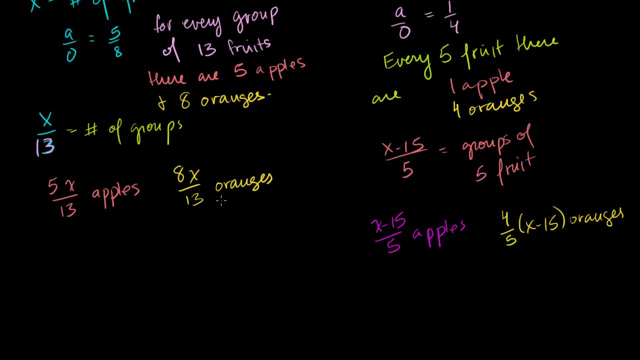 Now, what doesn't change? I'm messing with the number of apples, but I never changed the number of oranges, So this number, which is the number of oranges we started off with, has to equal this number, the number of oranges we ended up with. 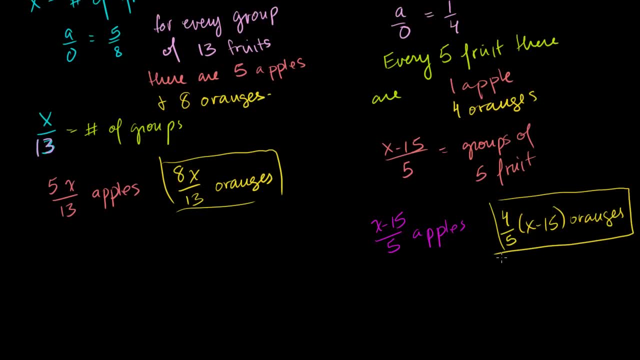 There's many ways to do this problem, but this is the way that's popping out at me. that might be straightforward, So let's see if we can solve for x. This has to be equal to that. That never changed, So I can use 8x over. 13 is equal to 4 fifths. 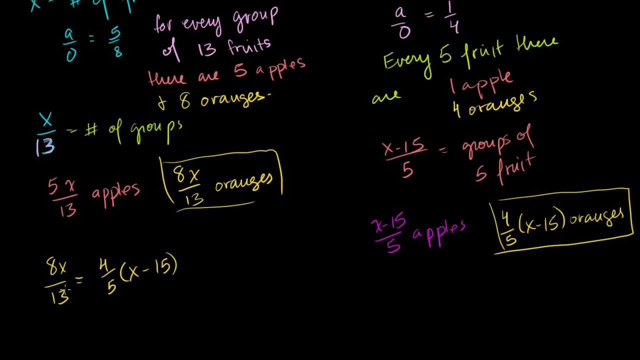 times x minus 15.. And maybe the best way to do this, let's multiply both sides of this equation times 5 over 4.. So it's times 5 over 4.. 4 times 5 over 4.. These cancel out. 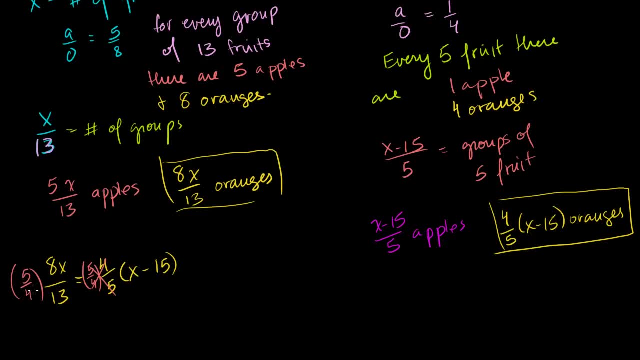 That just becomes 1.. What does this become? This becomes, you see, you get a 4 divided by 4.. You get a 2 there. This becomes 10x over 13,, that's, the left-hand side is equal to x minus 15.. 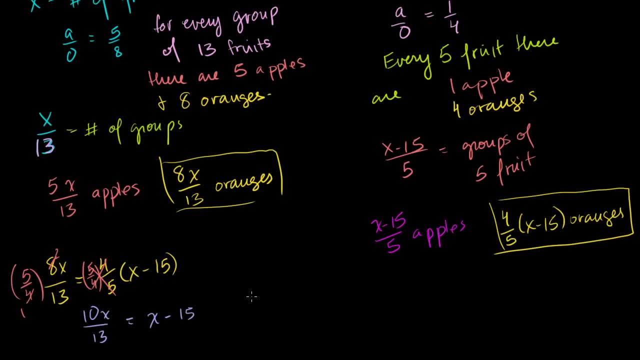 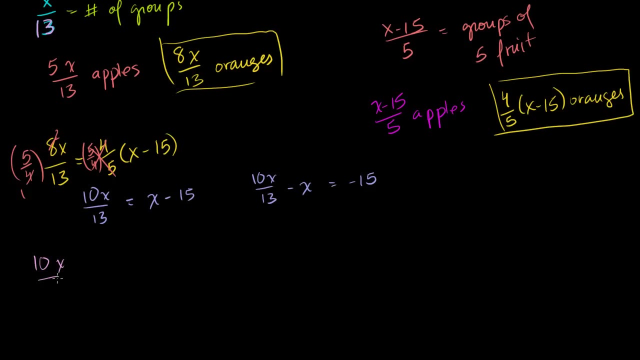 Now let's subtract x from both sides and we get 10x over 13. minus x is equal to minus 15.. Let me scroll down a little bit. And so what is this? This is the same thing as 10x over 13 minus 13x over 13..